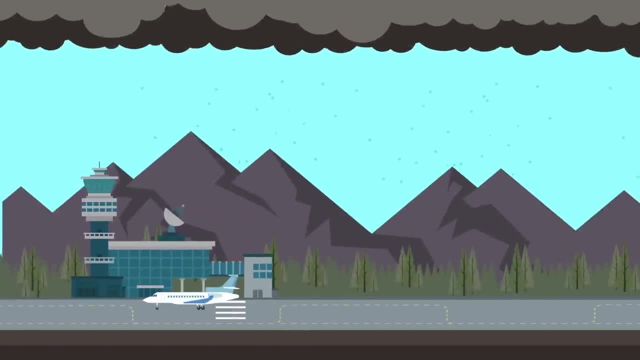 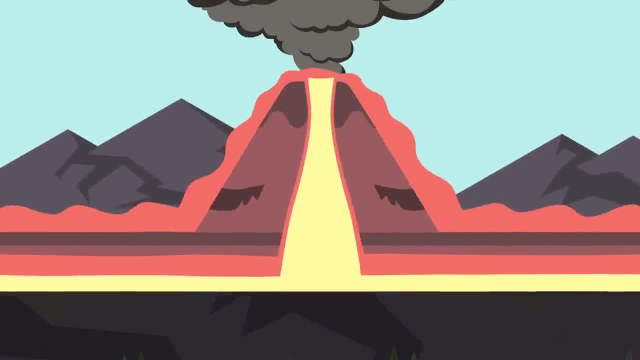 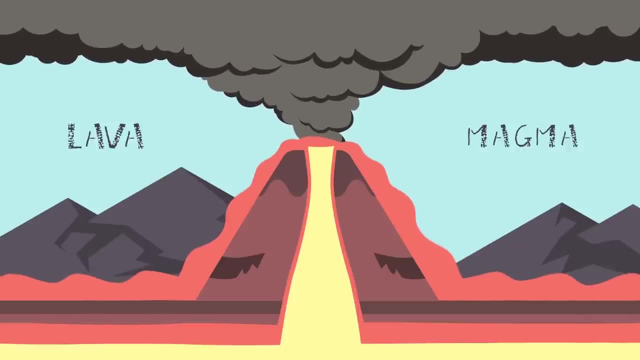 Bali airport to be temporarily shut down. What is the hot red fluid that comes out of an erupting volcano called? Is it called lava or magma? The correct answer is lava. Many people use the terms lava and magma interchangeably, but there is actually a clear distinction. 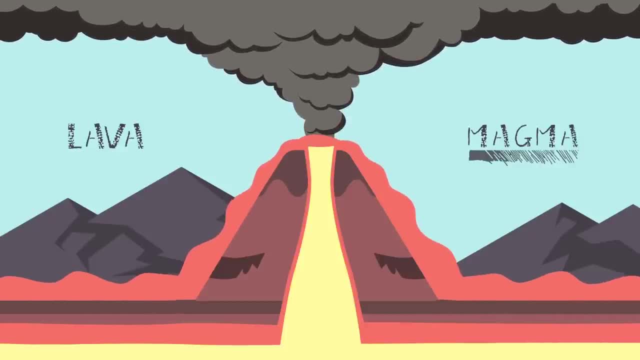 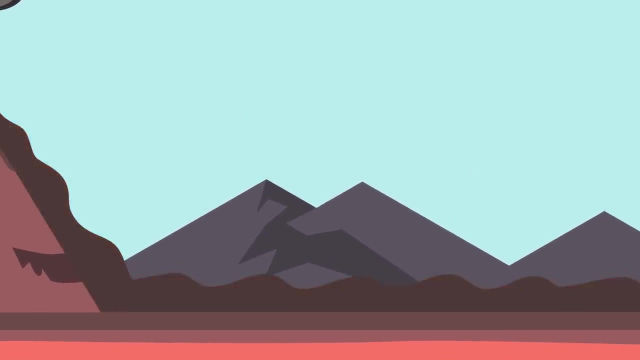 Molten rock that is still underground is called magma and the same fluid is called lava. when all the volcanic gas passes deep and it is flowing on the surface after a volcanic eruption, What happens when this hot lava cools down? If the lava spreads across a wide area, it hardens and small amounts turn into rock. 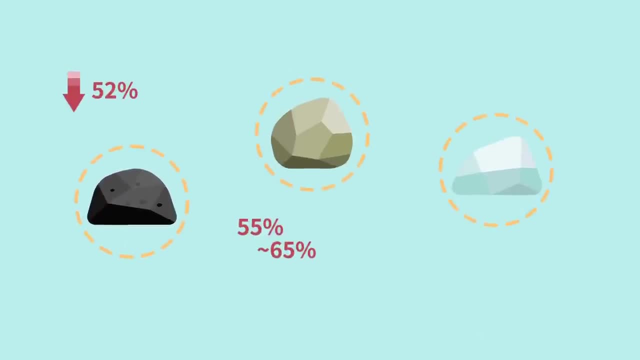 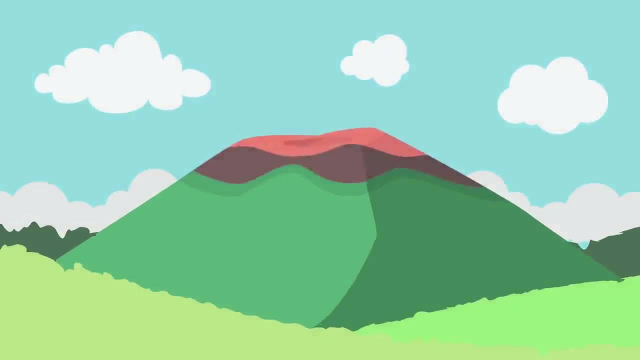 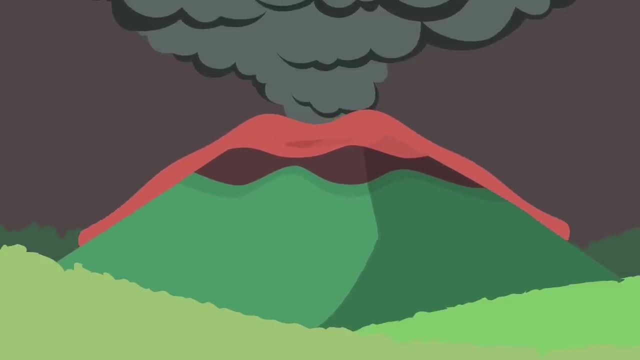 This volcanic rock is classified as basalt, andesite or rhyolite, depending on its silicon dioxide content. The basaltic lava of Mauna Loa in Hawaii has a low gas content and flows quietly. Basaltic lava can only reach the surface if there is a crack in the earth's crust. 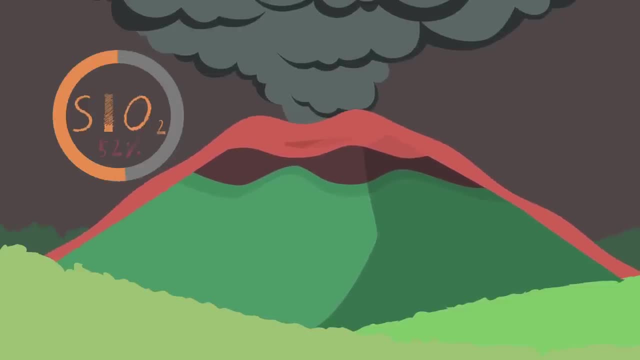 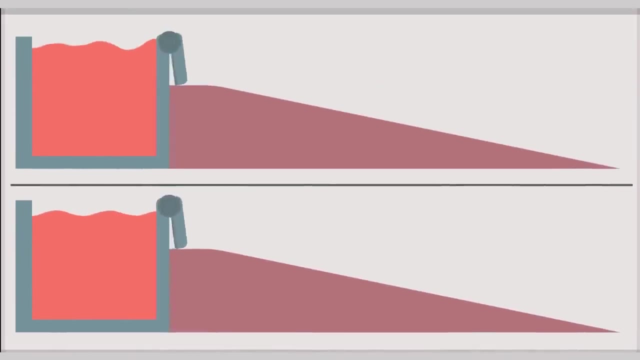 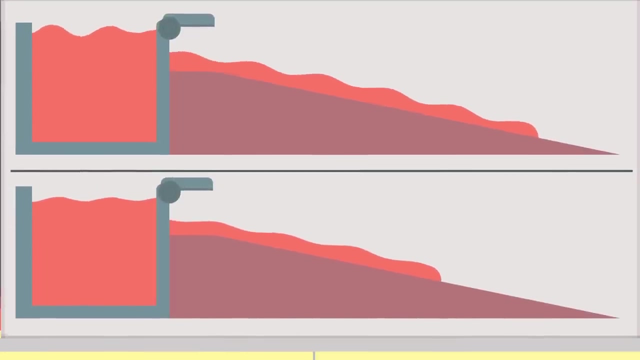 This type of lava has a silicon dioxide content of 52% or less, making it highly fluid with a low viscosity. Fluidity is a measure of how well a material flows and viscosity is a measure of how sticky it is. They are opposites of one another. 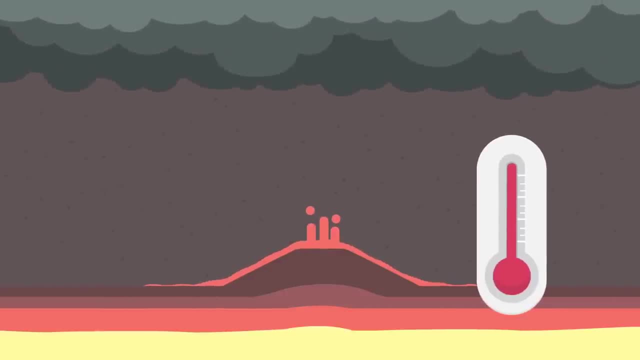 Basaltic lava has a high temperature and creates quite a lot of water. The basaltic lava has a high temperature and creates quite a lot of water. The basaltic lava has a high temperature and creates quite a lot of water. Pol Code provide a high amount of water compared. 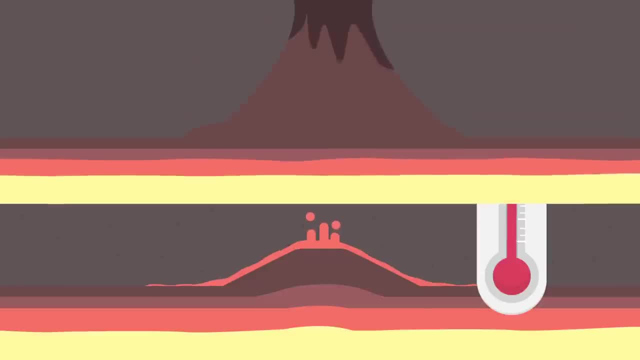 to the basaltic lava of South Korea. Volcanoes try to create fewer caves or kiwi, blamed on their exhaustive nature relative to amount of oxygen and ernst water characteristics. For instance, basaltic lava in the spring sea in Forum variant has many feminine stones. 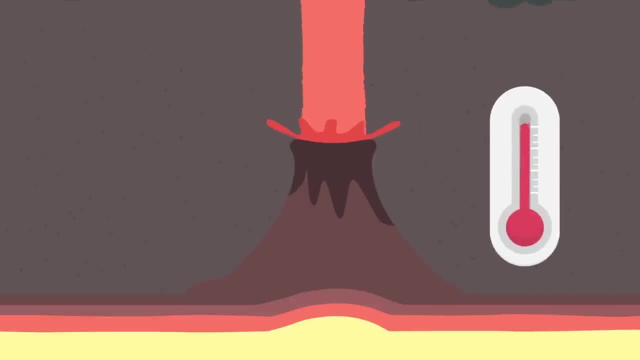 and the fit of basaltic lava is rescue-worthy Filet of어 companions can also unique. writer of basaltic lava in福주, just below In July, Yoon Dong-ah, new graduate major in relations with drawn to be The former municipal leasehold. 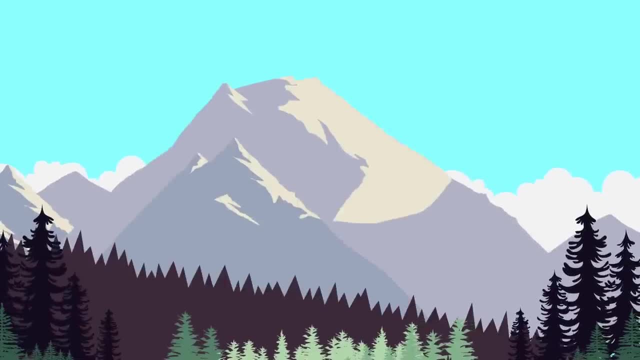 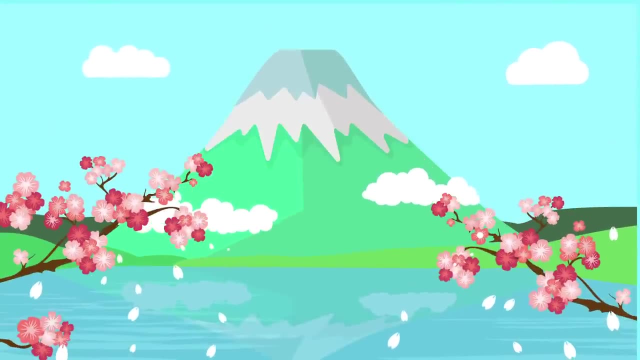 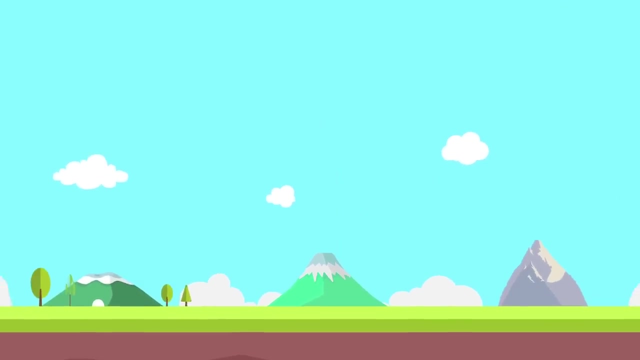 Auntie psychology Do Над that the solar network has Characteristics of andesitic lava. volcanoes like Mt Fuji in Japan are somewhere between basaltic and rhyolitic lava volcanoes. Earthquakes are another disaster caused by volcanic or fault activity. 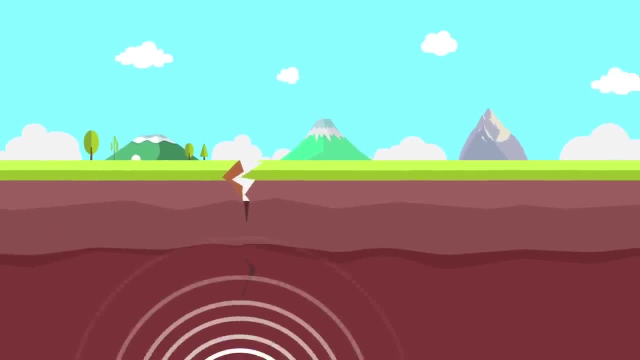 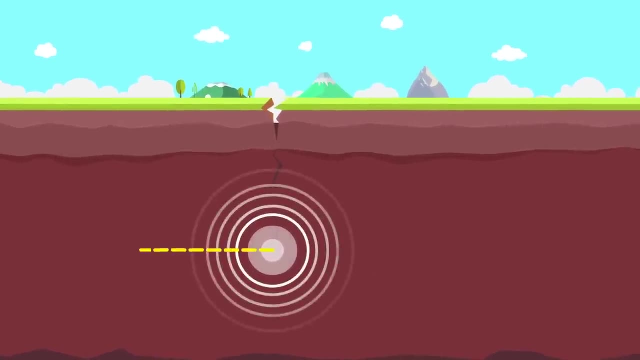 In an earthquake, the energy built up inside the earth is released in all directions in the form of waves, causing the ground to shake. The point inside the earth where the earthquake has occurred is called the focus, while the point on the surface directly above the focus is called the epicenter. 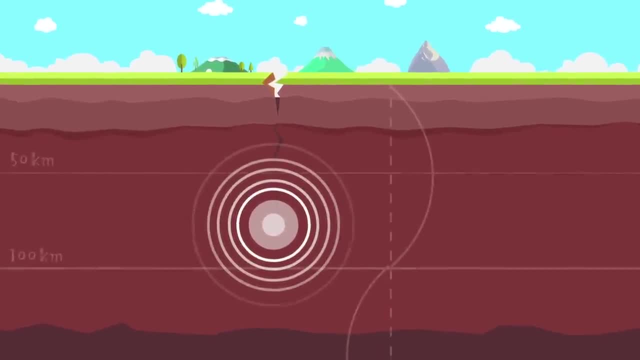 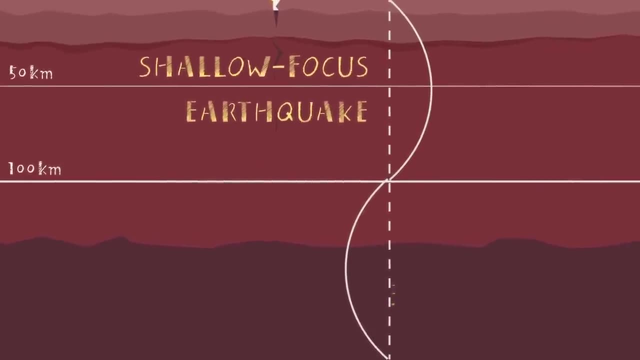 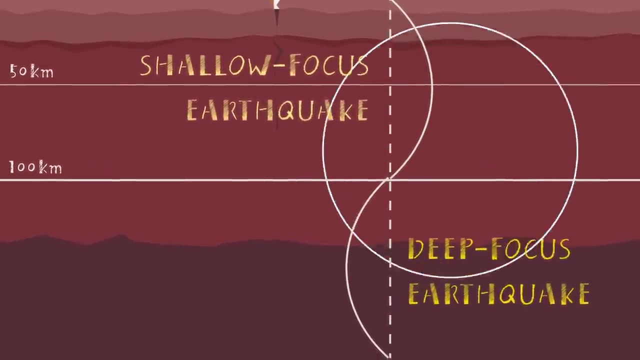 Earthquakes are classified according to the depth at which they occur. An earthquake whose focus is less than 100 km deep is called a shallow-focus earthquake, and an earthquake with a focus deeper than 100 km is called a deep-focus earthquake. The waves caused by an earthquake are called seismic waves. 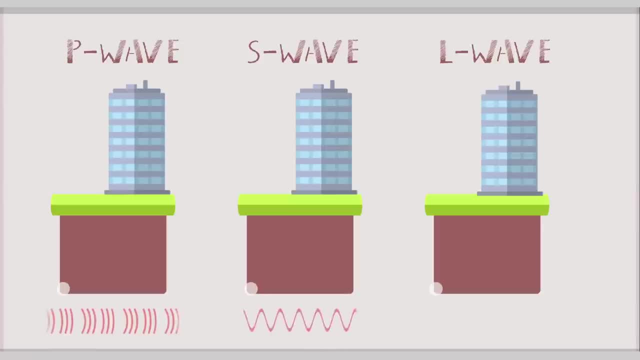 There are three types of seismic waves: P waves, S waves And L waves, The fastest of which are P waves, followed by S waves and L waves. The amplitude and the amount of damage caused by earthquake are expressed in the opposite order. 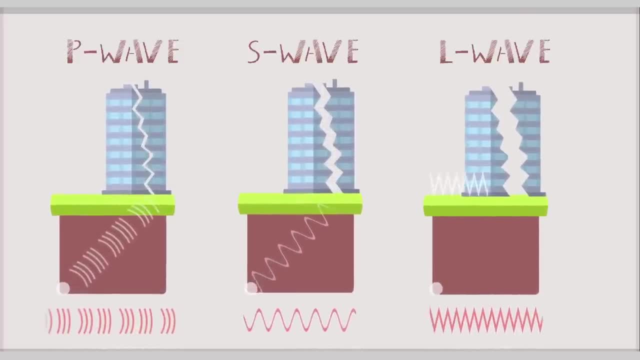 L waves are the most destructive, followed by S waves and P waves. Naturally, stronger amplitude results in more damage. Given the same underground conditions, amplitude and damage increase together. There has just been an earthquake. The red house is closer to the epicenter than the blue house. 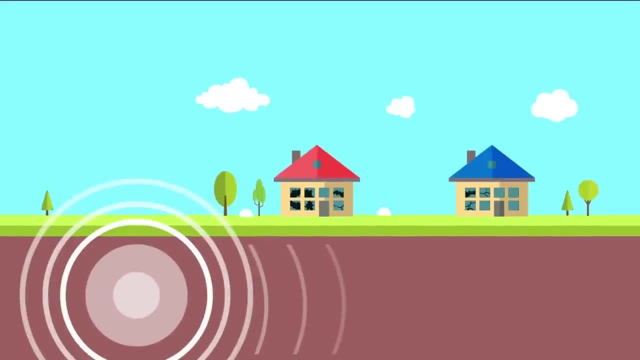 As a result, more windows in the red house were shattered. In other words, the seismic intensity of the earthquake was greater at the red house. Seismic intensity is a term used to describe the strength of earthquake vibrations and how much damage they cause. 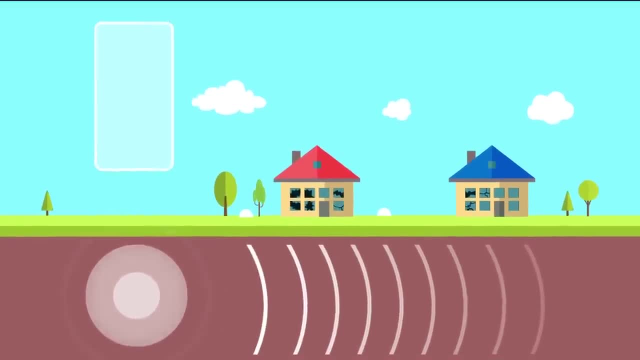 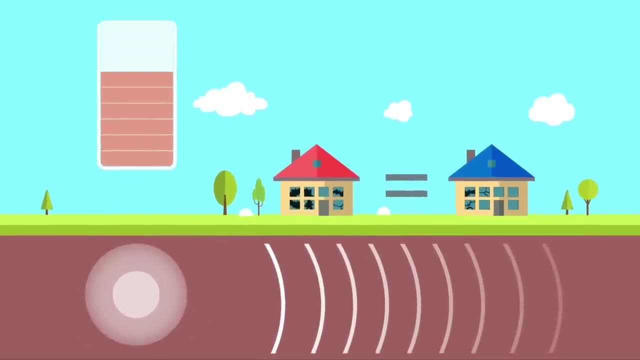 However, the amount of energy released by the earthquake is the same at both the blue and the red house. Magnitude is a numerical value that represents the amount of energy released at the focus, rather than at the focus at the focus of the earthquake. 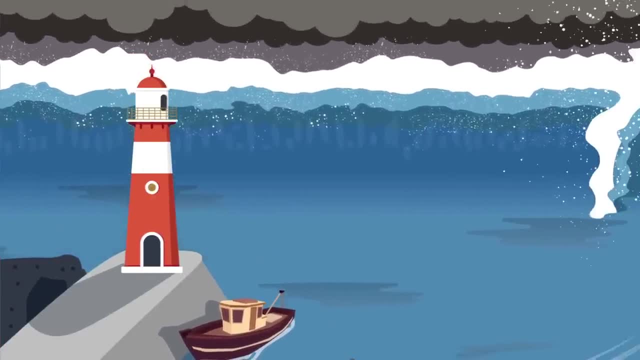 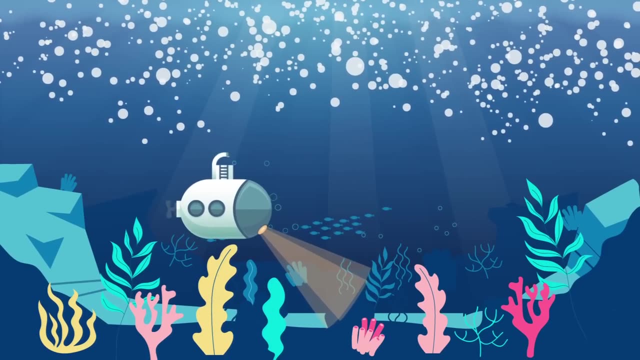 There is another type of disaster we should mention at this point. Many of us remember the Japanese earthquake of 2011,, which demonstrated the power of seismic sea waves. These seismic sea waves are caused by sudden changes in the crust due to undersea earthquakes. 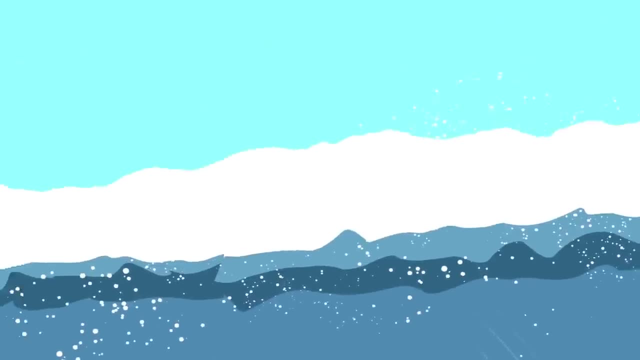 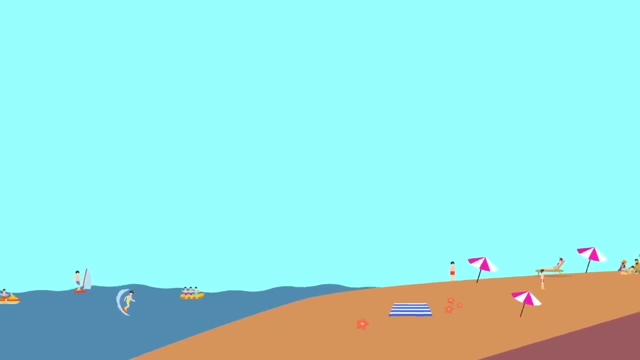 or volcanic eruptions. These seismic sea waves are also called tsunamis. When we're at the beach, it's easy to see that the water gets shallower as it gets closer to the shore. Likewise, the depth of seawater decreases as a seismic sea wave approaches the shore. 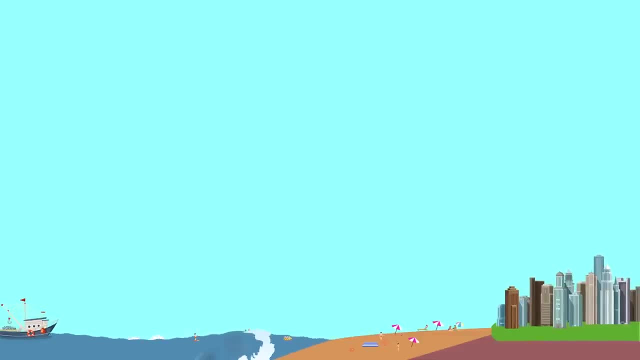 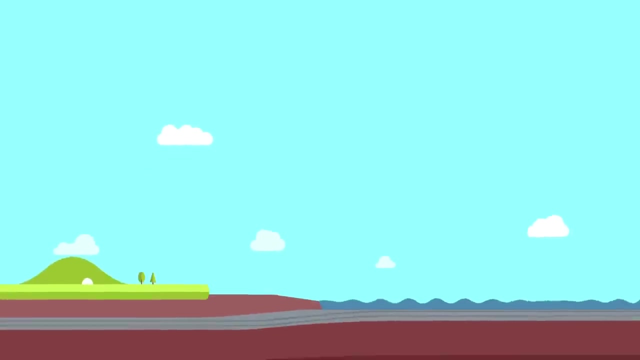 As the wave approaches, it moves slower, but the height of the wave increases. That is why, as we see in many disaster movies, seismic sea waves grow taller as they approach the shore. Where do these powerful underground forces come from? As we've already mentioned, the ground we stand on is the surface of the ocean, and 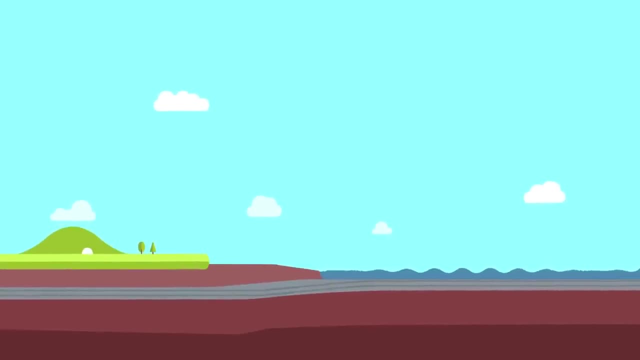 the sun is always moving. Below the crust on which we live is the Earth's mantle. The 100-kilometer-thick layer of solid rock, including the crust and part of the upper crust, is called the lithosphere. The upper mantle that lies beneath the lithosphere is called the asthenosphere. 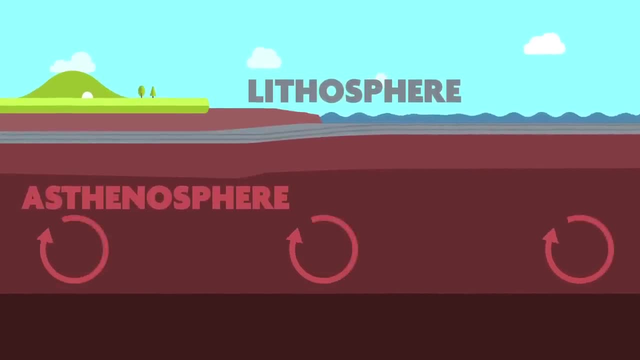 The asthenosphere is also solid, but the rock here is softer due to high pressure and high temperatures. Differences in temperature between the inner and outer parts of the asthenosphere allow convection to occur. This is the reason why the Earth's mantle is so solid. 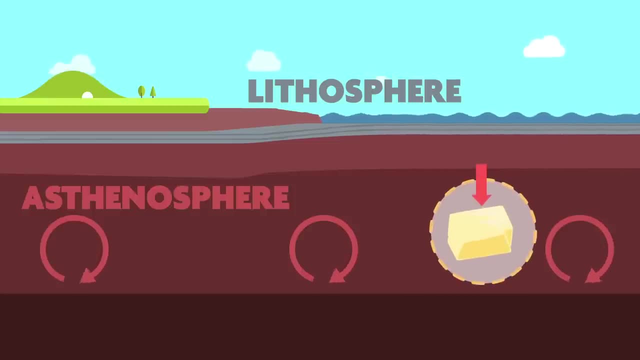 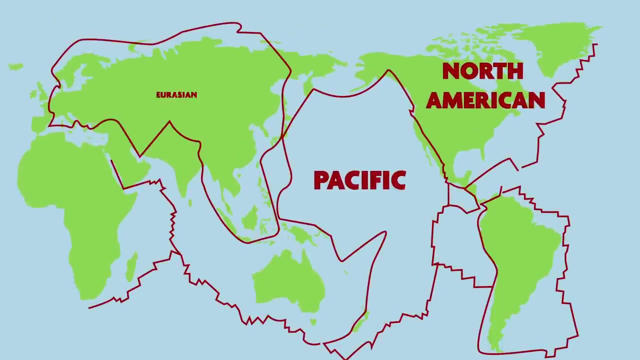 In some ways, the consistency of the asthenosphere can be compared to that of butter: Even though it is a solid, it can be pressed and molded. Convection in the asthenosphere forms the foundation of plate tectonics. The Earth has 10 small and large plates, which include the North American plate, the Pacific, 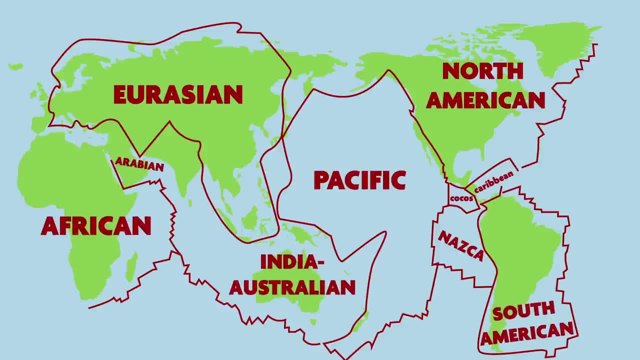 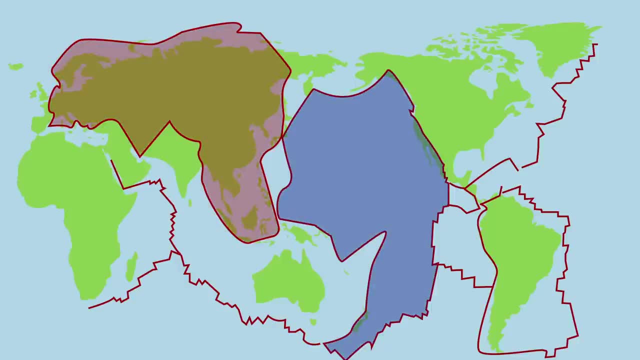 plate, the Eurasian plate and the Nazca plate. The Pacific plate is an example of an oceanic plate and the Eurasian plate is an example of a continental plate. The relative motion of these plates causes the Earth to move. The motion of these plates causes crustal movements such as earthquakes and volcanic. 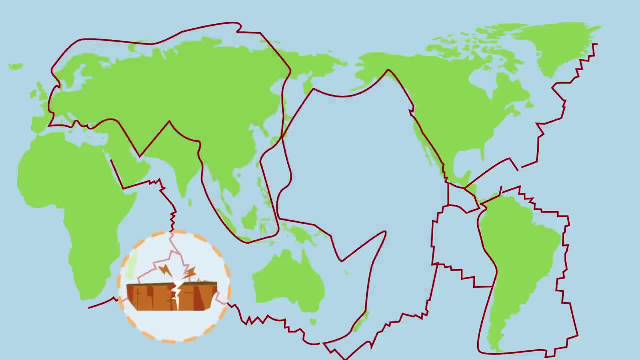 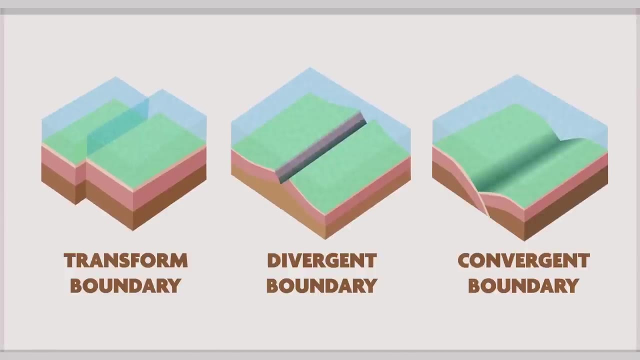 eruptions at plate boundaries. 90% of Earth's earthquakes and 75% of its volcanic activity occurs in what is called the ring fire. There are three types of plate boundaries: Transform boundaries, divergent boundaries and convergent boundaries. 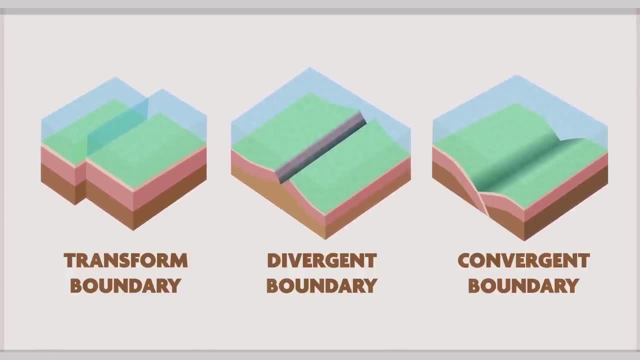 In a transform boundary, two plates move horizontally to one another. In a divergent boundary, the plates move horizontally to one another. In a divergent boundary, the plates move horizontally to one another. The plates move away from each other, while in a convergent boundary the plates collide. 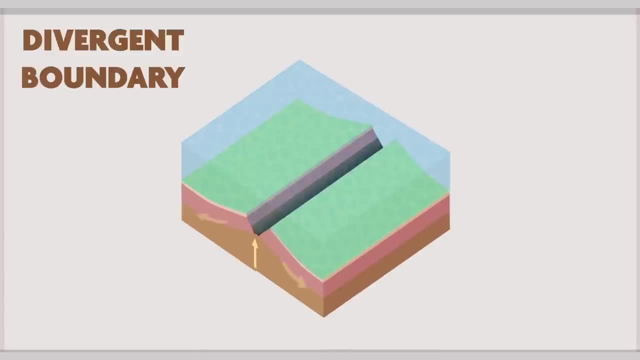 Divergent boundaries are the result of rising convection currents in the mantle and are characterized by volcanic activity and shallow focus earthquakes that occur at relatively shallow points. Divergent boundaries also create V-shaped rift valleys and undersea mountain ranges. Iceland is an example of an undersea mountain range that has been pushed above the ocean.